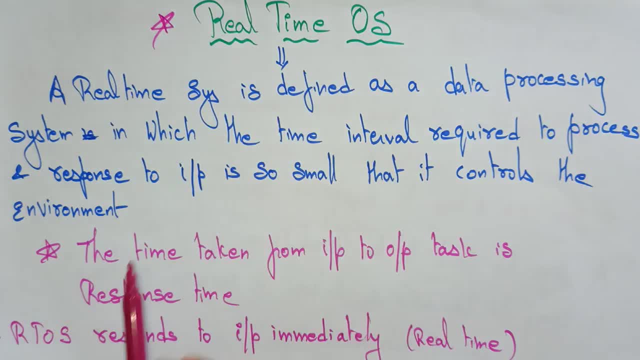 real time operating system. So by reading this name what you are understanding, we are using these type of operating system in the real time applications. So some real time applications. that means whenever we are given the input, we have to get the output very quickly. So input whenever. 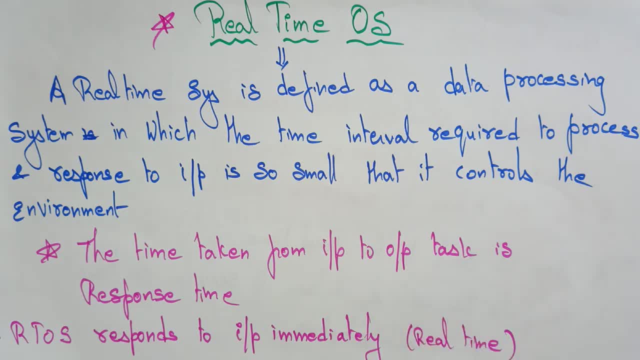 you are given the input, you have to receive the response immediately. Those you call it as a real time means these type of response. you call it as a real time, So in those applications we are using a real time operating system. So let's have a look on this. what exactly the real time? 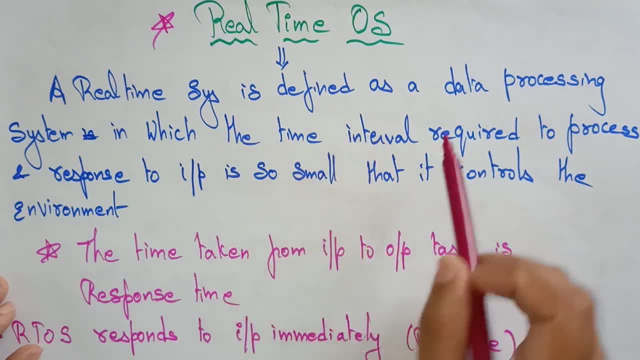 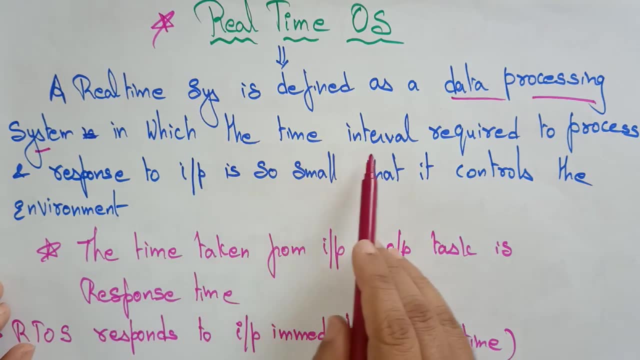 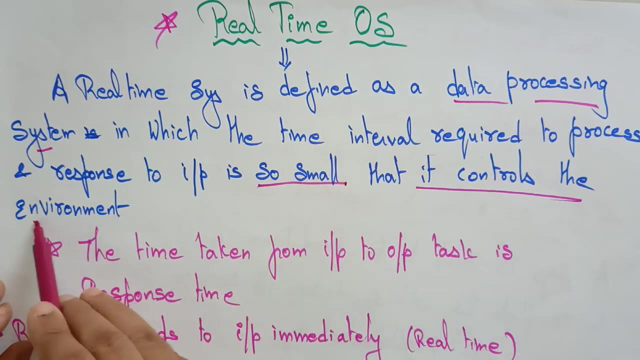 operating system is A real time system is defined as a data processing system, So it is a one of the concept. it's a data processing system in which the time interval required to process and response to inputs is so small that it controls the environment That is. 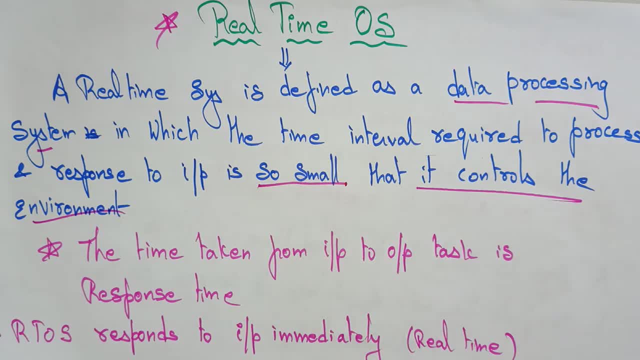 what I said. So whatever the input we are given, it has to respond very quickly. So the interval between the processing, the input, and output is very small, is so small the response. it should be very small So that it going to control the environment. 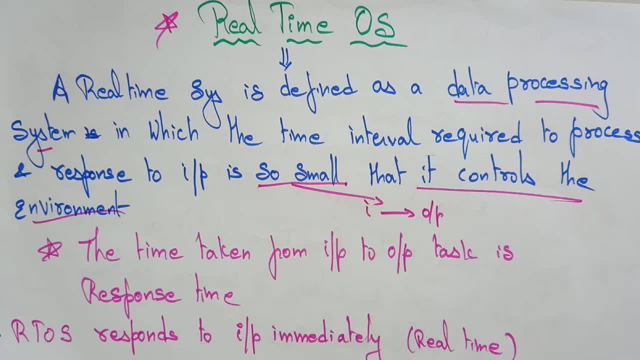 Suppose, if you take your artificial intelligence, like if you take the automatic car, So the automatic car it is already. means without the driver. So whenever you are given the instructions, it is going, it will take you to the destination. So without the driver. So there we are, using the real time operating system. So here that it going to control the environment Whenever we need to. a person is coming means whenever it feels some sense, or 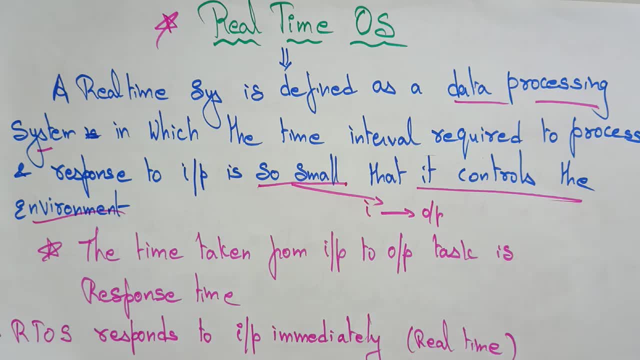 with the help of the sensor, it feels something is going to be come in front of the car, So it applies the brake automatically. So if it doesn't apply in the real time, obviously the car is going to hit the person or something like a thing, anything, Okay. So the input and output response should be very small. The time interval required to process and response is very small, So that it going to control the environment. So I hope you understand what exactly the real time operating system is. 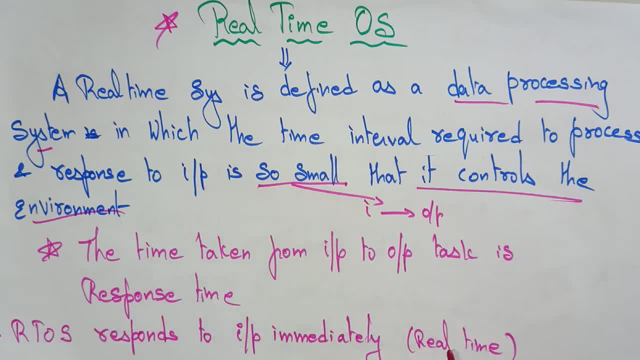 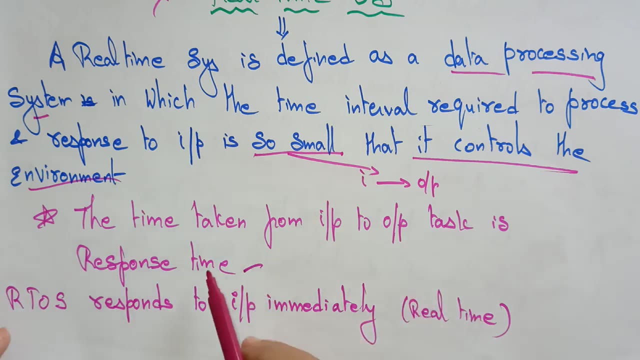 Another example: you can take the traffic signals. the traffic signals, Okay. So whenever the green light and red light or an a low light, everything is depends upon the real time operating system. Okay, The time taken from input to output task is response time. What exactly the response time? response time means whenever I say something, if you respond immediately. So the time between I asked the question and you're replying, So I'm asking the question and you're replying. 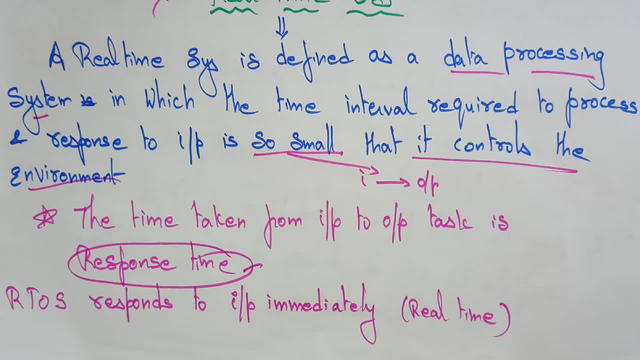 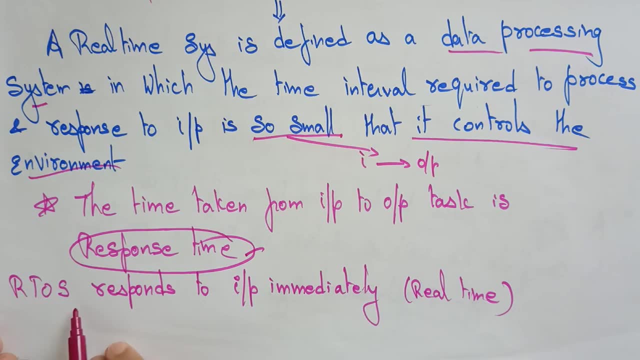 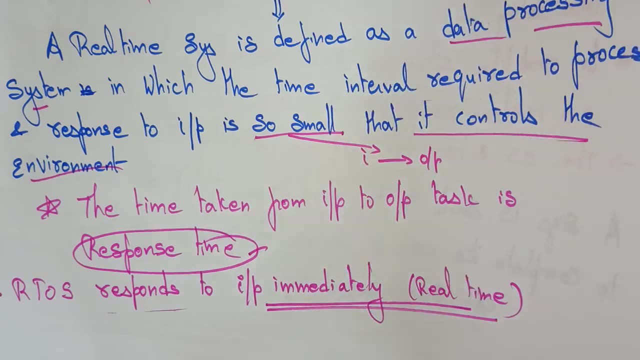 and you are replying, so the time in between, whatever it takes that, you call it as a response time. The time taken from input to output task is response time. The real-time operating system responds to input immediately. So whenever it is responding immediately, then you call it as a real. 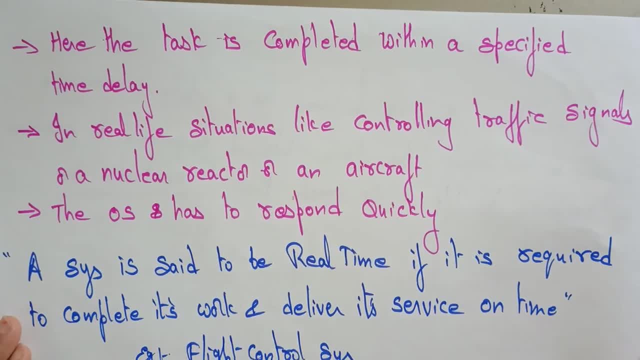 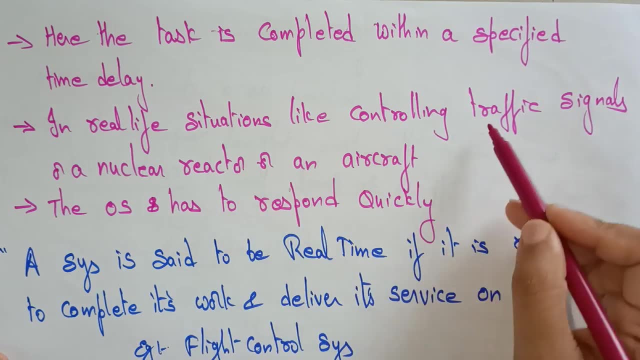 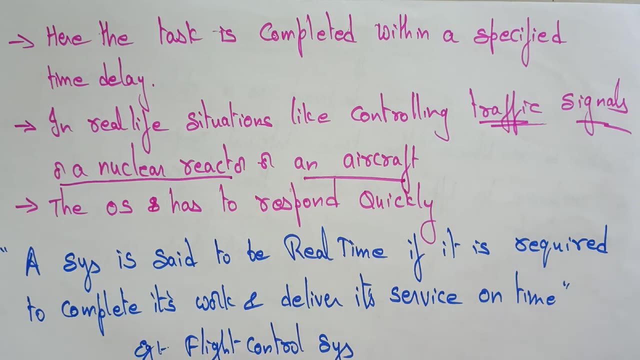 time. Here the task is completed within the specified time delay In real-time situations like controlling the traffic signals or nuclear reactors or aircrafts. so in all these fields we are using this real-time operating system. so which is going to control the traffic signals in? 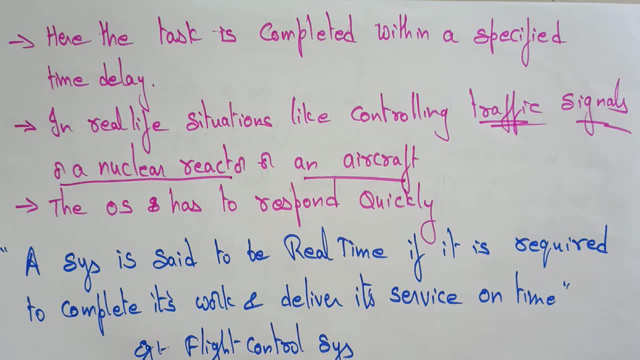 the real-life situations If you use a nuclear reactor or if you use an aircraft, everything should be response in a real-time applications. So the input and output- it's a response time of input and output- should be very small. It should be response time of input and output should be very small. It should be response time of input and. 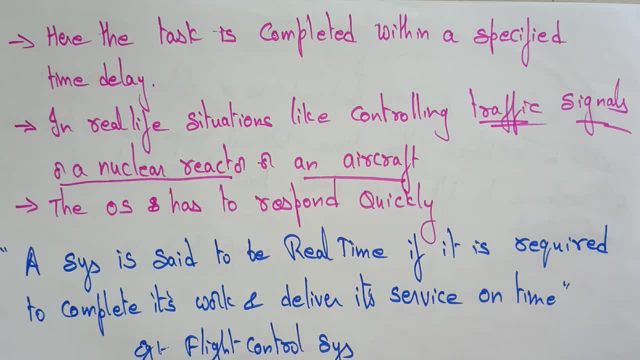 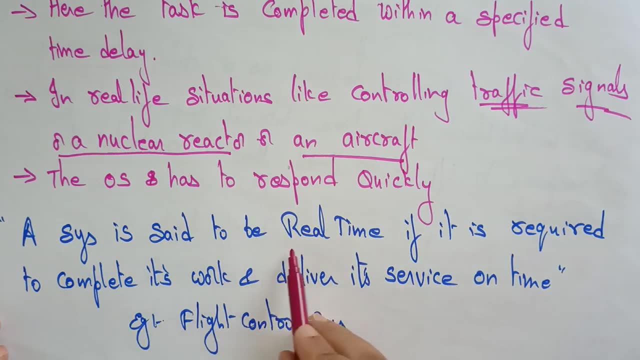 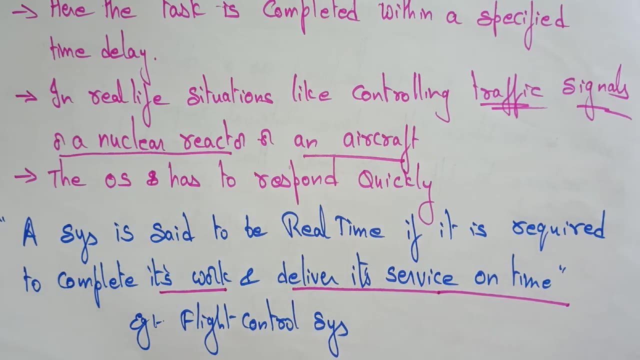 immediately. whenever you are given the input, it has to respond immediately. the operating system has to respond quickly. a system is said to be real time if it is required to complete its work and deliver its service on time. okay, so this is exactly the definition of the real time a system. 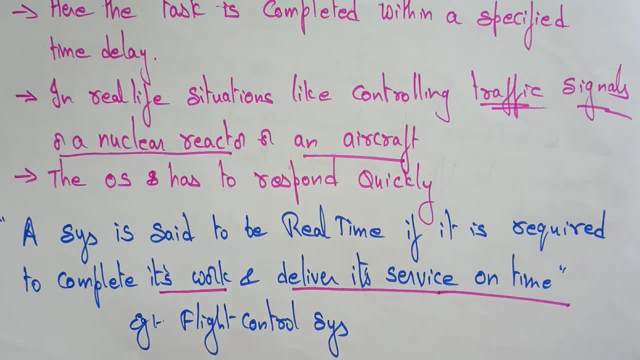 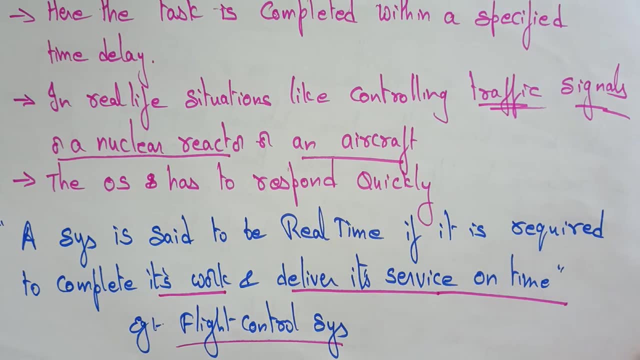 is said to be real time if it is required to complete its work and deliver its service on time, like the flight control system. so the flight control system, whenever you are operating the flight control means it has to respond whenever the input is given. okay, otherwise the flight we. 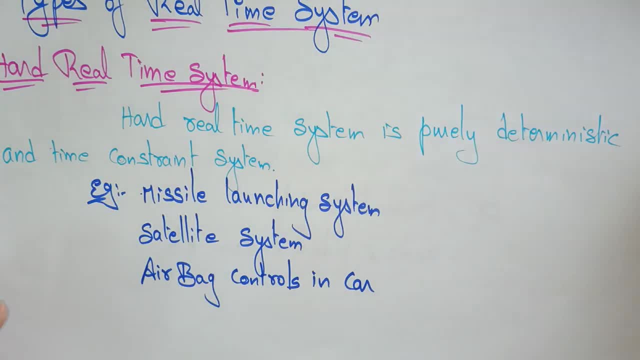 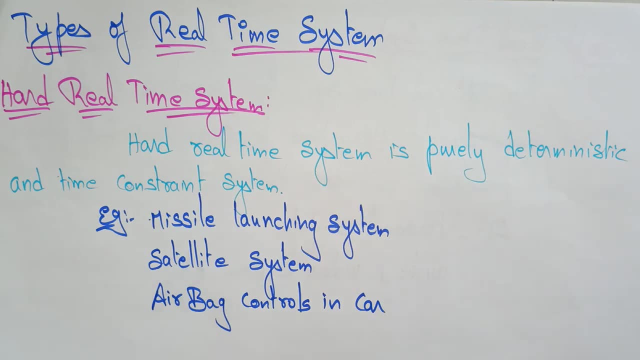 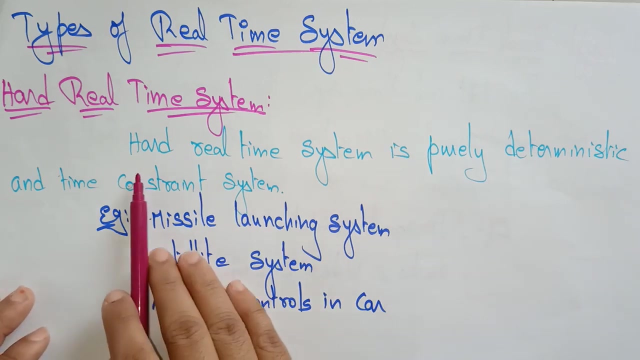 may crash. let's have a look on the types of real time systems. actually, there are two different types of real time systems. one is the hard real time and one is a soft real time. okay, so what is hard real time and what is a soft real time? let's have a look on this. the hard real time system. 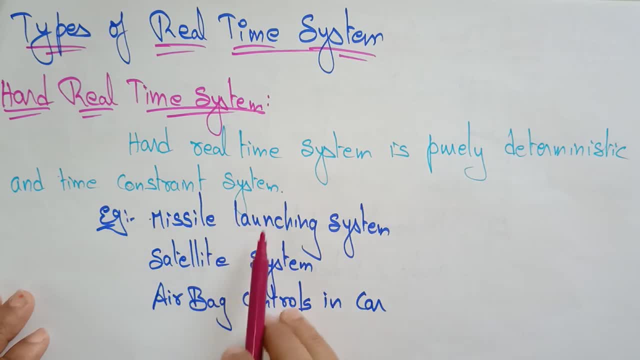 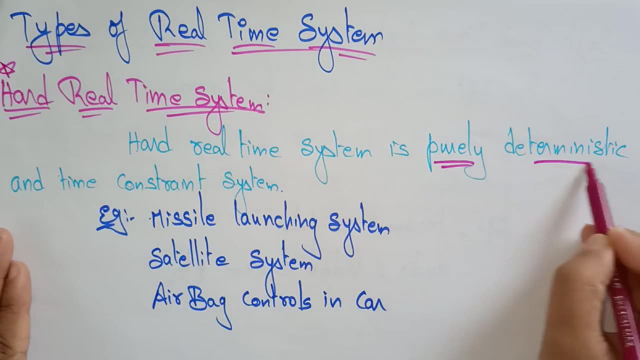 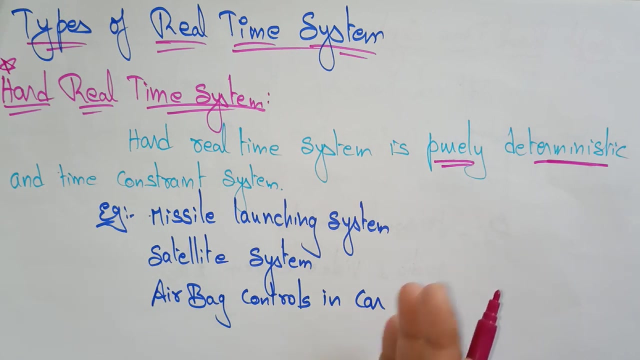 is purely deterministic and time constrained system. so here what exactly the hard real time system means. it is purely deterministic, means and some time constrained system should be there. so within that a many time time it has to respond quickly. it's purely deterministic, okay, like missile launching system, satellite system, airbag controls in car. so everything should be respond. 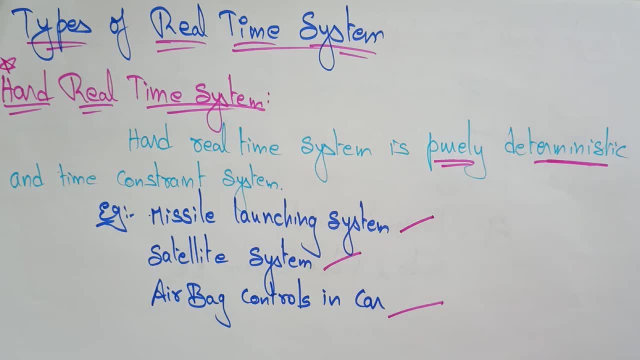 immediately airbag controls in car how it is going to be. whenever the car is going to kick something, it's very hard. if you keep the seat belt, it's automatically within a seconds it has to open the airbag control. okay, airbags has to be controlled in a car whenever something is. 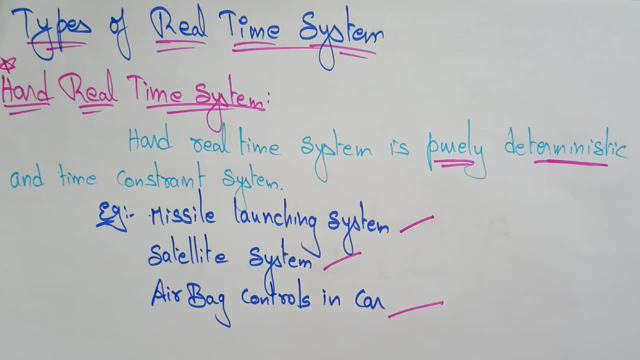 going to be hit hardly. okay, that is a hard. real time system mean it has to be performed immediately means without any delay. it's a missile launching system is also like that. whenever you just click on that missile launching, it has to be go and it has to be crack. 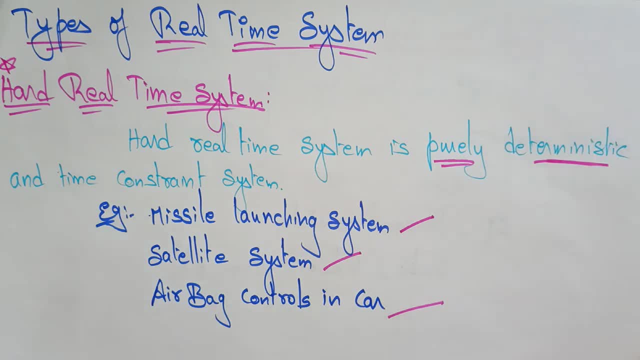 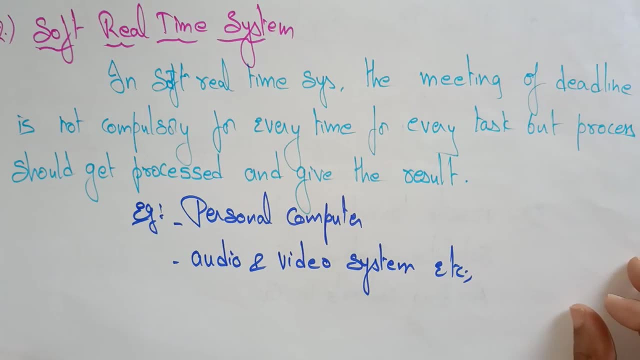 okay, just like a satellite system. so these are all you call it as a hard real time system. then what about the soft real time system? maybe it has some delay. should be. avoidable means means acceptable, not avoidable, whereas in hard real system you are not acceptable. the 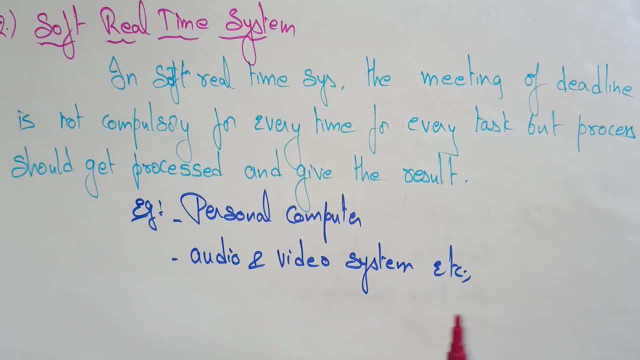 delays. but in the soft real time system it seems to be very soft. that means in soft real time system the meeting of deadline is not compulsory. this is the what i am talking about. the small soft real time system means the meeting of the deadline is not compulsory for every time, for every task. 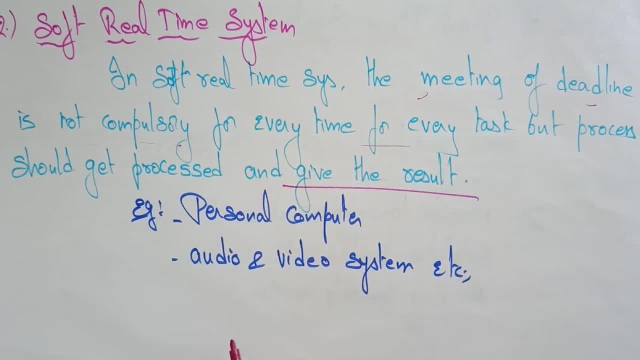 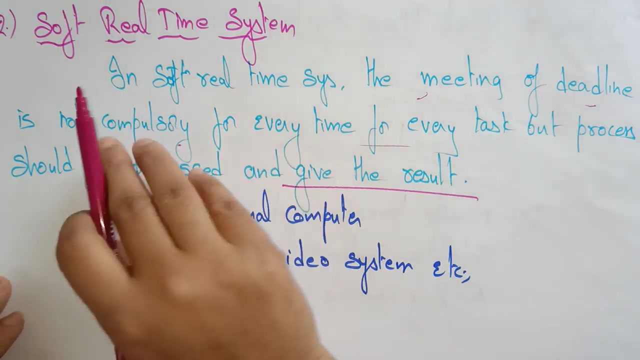 but process should get processed at a given and gives the result. so anyhow it gives the result but there is not compulsory. it has to meet. the deadline means within this time it has to be completed. there is no that much of uh criteria in the soft real time. that's why we have to. 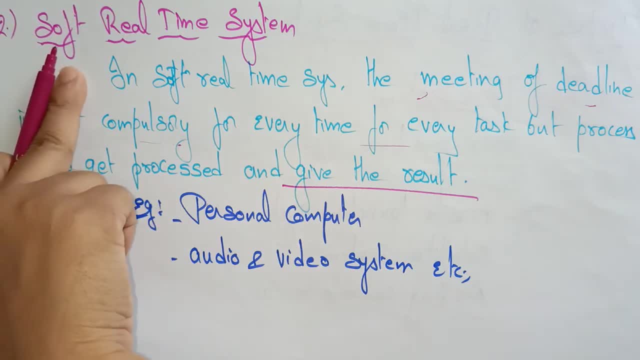 call the name itself is a soft. soft means it has to take some time to complete the work. okay, but the task is it has to complete the process and gives the result. i i won't get. i want the result, but i am not giving any deadline to that. okay, so anyhow, but not taking lot of time.